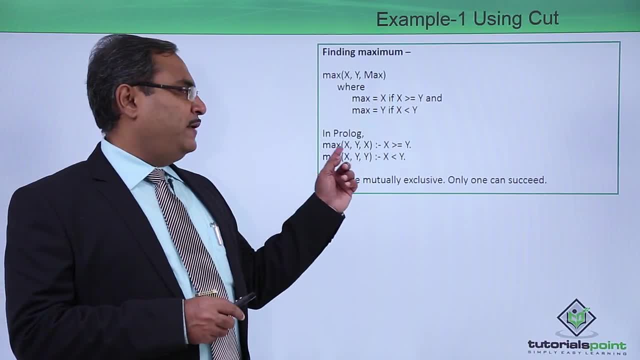 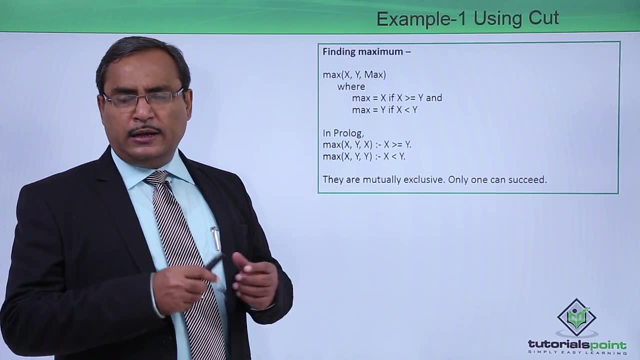 then this is true. So I should not go for checking both of them, because if it is true, then this is true. condition cannot be true. So that is why if I write in this simple way in prolog, then all the clauses are going to get executed and ultimately, obviously, I shall get the correct answer. but here 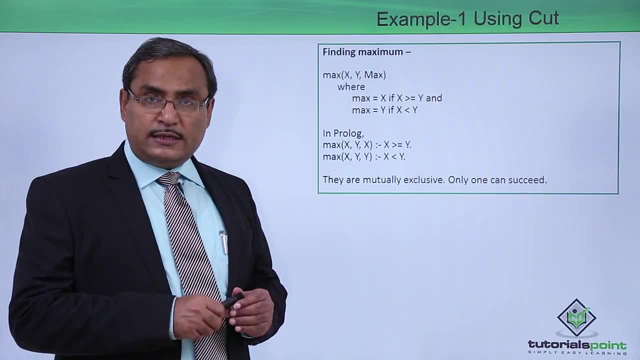 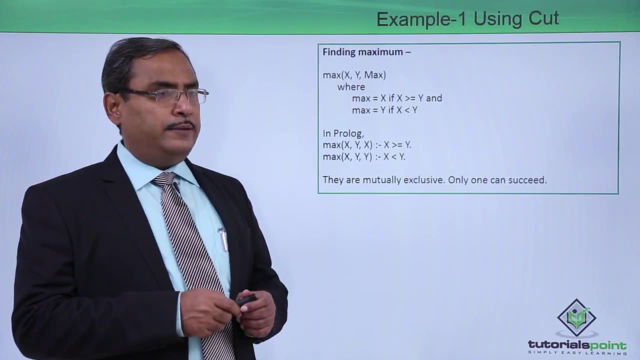 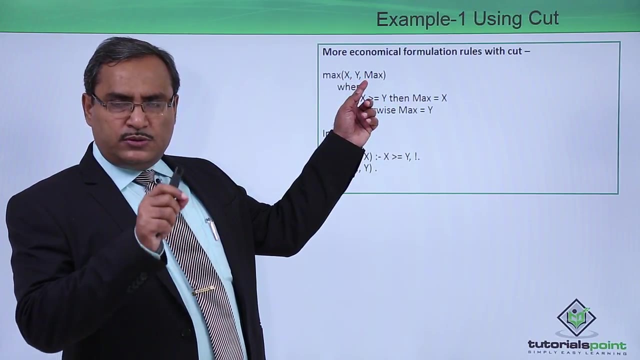 all the clauses are getting tested. So that is why let us use cut to prohibit this backtracking. So let us change our algorithm accordingly, So max x, y will be equal to max. that means maximum of x and y variables will be kept in the max, where if x is greater than equal to y, then max is equal to x. 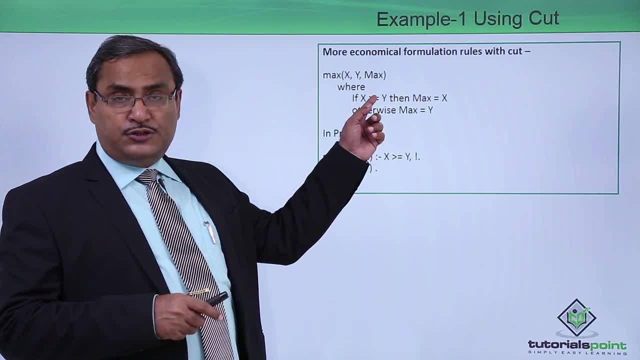 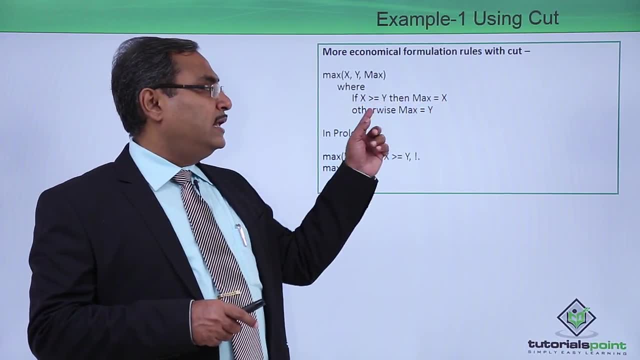 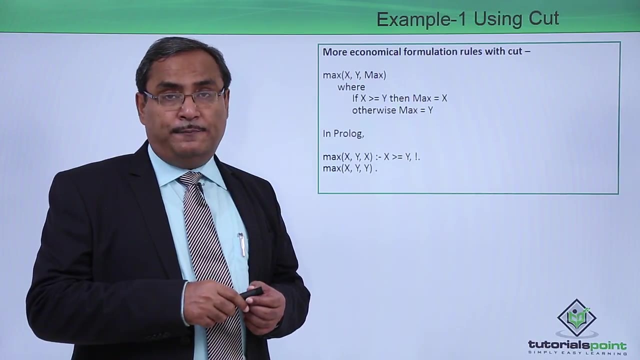 here you see it is. otherwise that means if it is true, then this part is not getting executed. So if x is greater than equal to y, then max is equal to x. otherwise max is equal to y. So if I write this algorithm in this form, then how to write the same in prolog? So max x and y are two input. 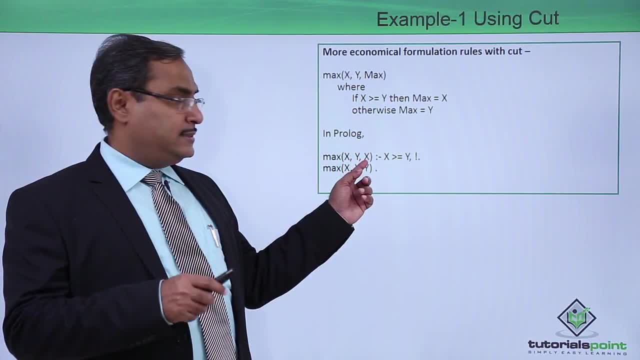 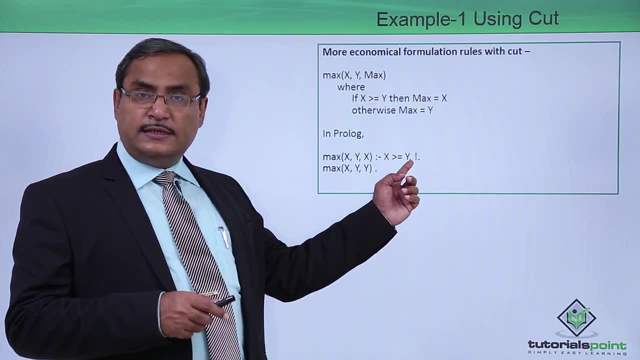 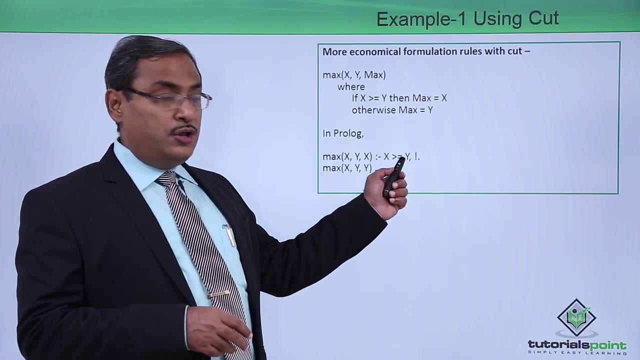 variables will produce x, the max in x. if x is greater than equal to y, cut this is and comma and this is cut. Cut indicates that, as the logic has crossed this one, if this condition is true, then obviously this particular clause is not going to be traced. 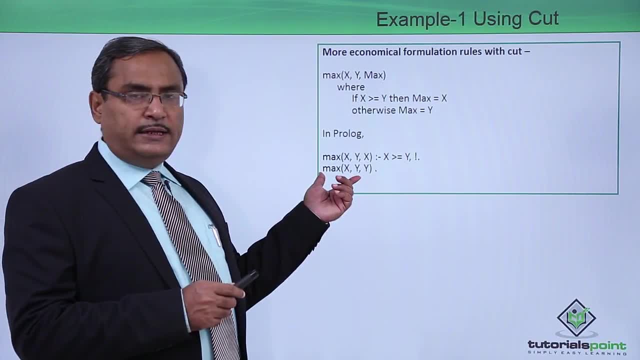 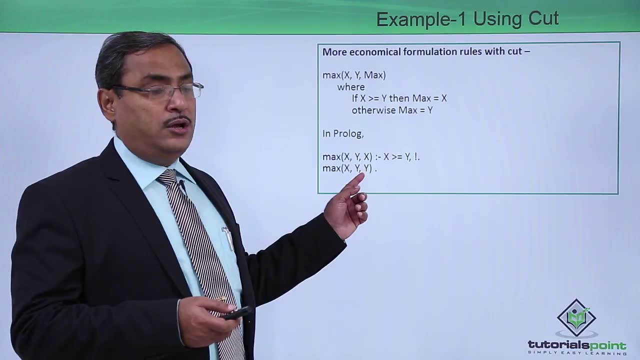 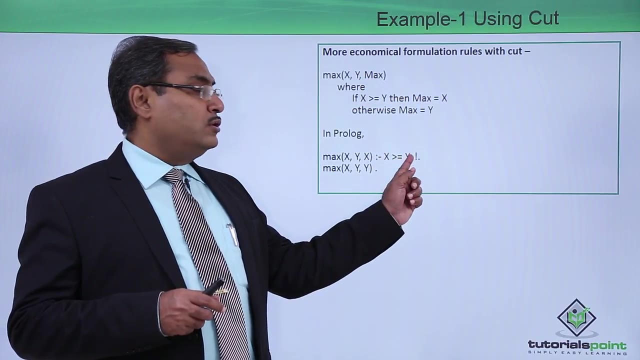 So that is a use of this cut. So otherwise we can write this one as x and y. the max will be y otherwise. So there, I need not to check whether y is greater than x or not. that is quite obvious, because when this condition is not true, then it cannot cross this cut. because here it is and 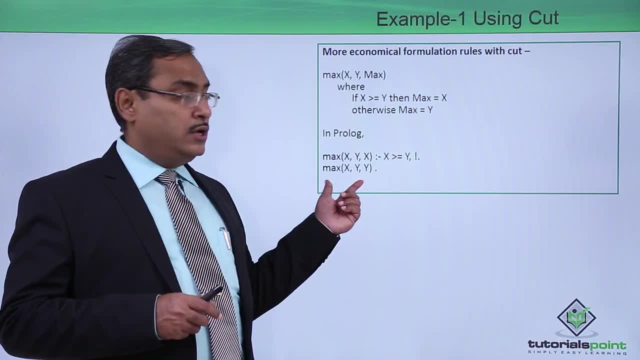 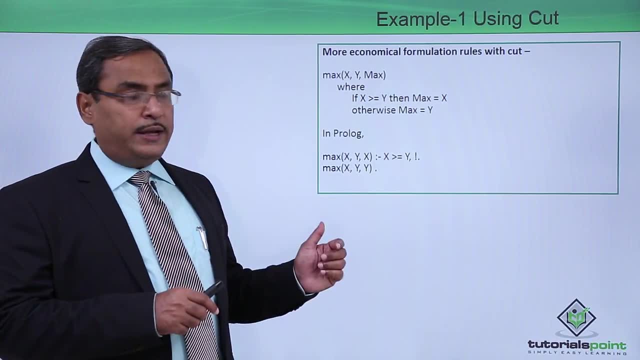 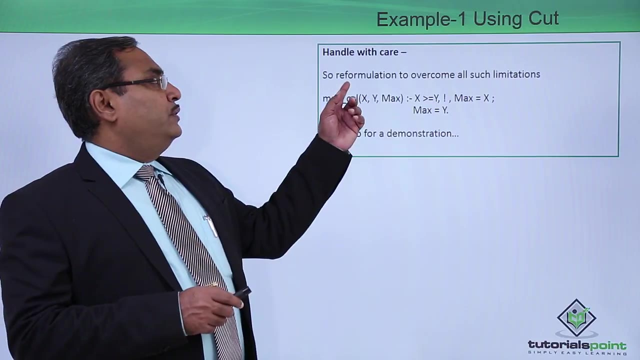 so if the first condition is false, then it will come to this clause execution, otherwise it will cross this cut and the backtracking will be prohibited. So in this way we can have a better logic in our prolog programming code. So for the reformulation. 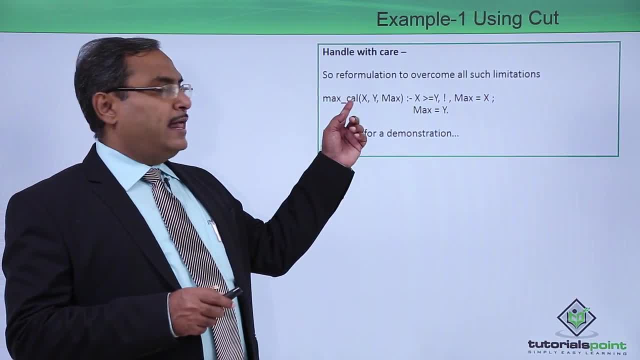 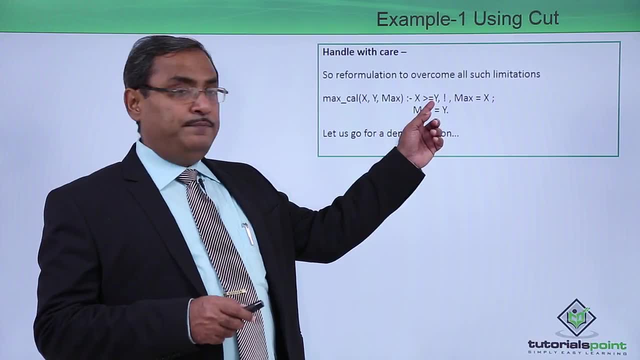 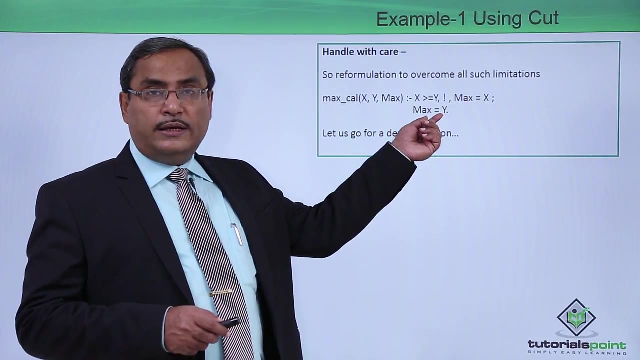 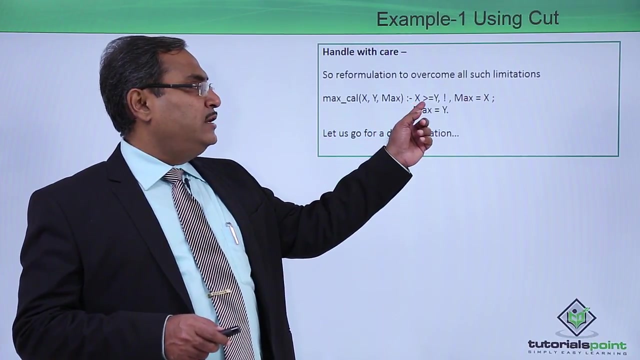 to overcome all such limitations. max cal x, y will initialize max accordingly. So if x is greater than equal to y, then cut max is equal to x. here it is semicolon means, or max is equal to y. So in the single clause I could have written the full story there. So if x is greater than 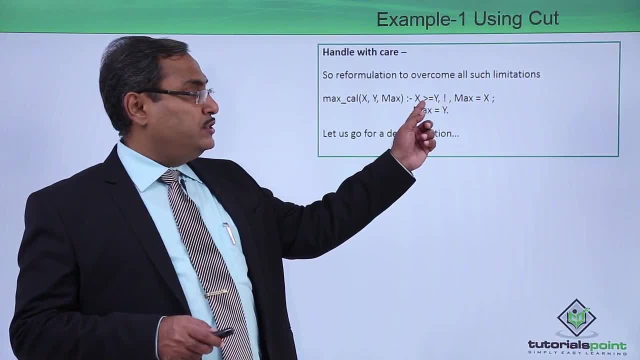 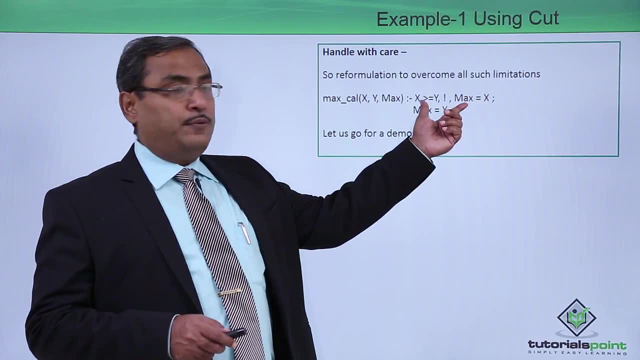 equal to y. cut. cut means if it is condition is true, then it will come to this part. Then obviously it will not go for this. or because if, in case of all logic, we know that if any one of the conditions is true, then output will be true in that case. Otherwise, if it is not, 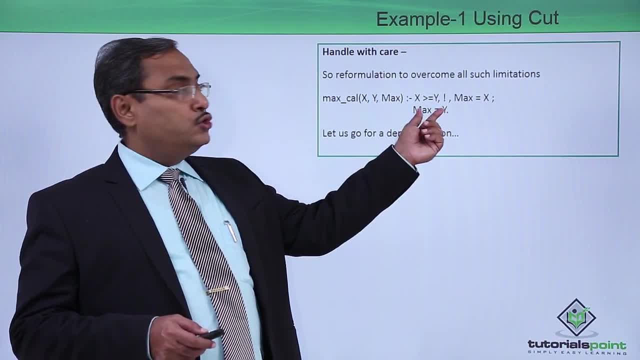 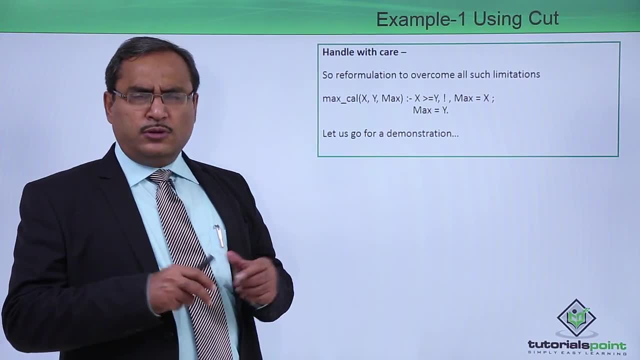 true, then it will come to this next part of the or. So in this way I shall be getting our maximum value of x and y in the variable max in this way. So let us go for the practical demonstration to understand whatever we have discussed right now. So here is the demonstration for you. 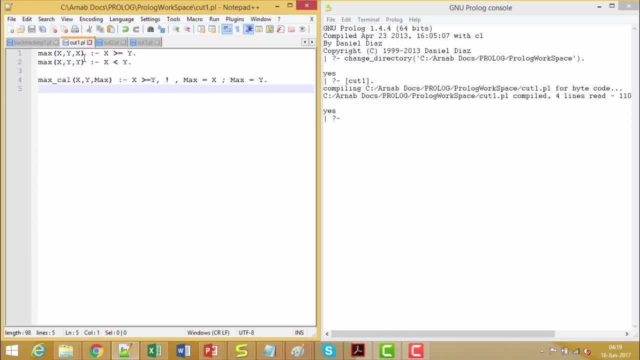 So here is the program and here we are having clause max and here we haven't used the cut symbol, that is exclamation symbol here. So let us see that. what are the difficulties we are having? So now, at first we have loaded this cut one dot pl, and also we have compiled without any error. 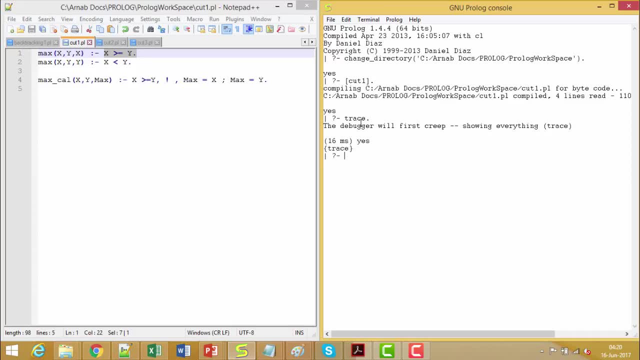 So I'm just making this press on and executing the code. Okay, so we have given value, that is, 200 and 100, and x will be the required maximum to be calculated. X is a variable here, So at first it is calling 200, 100 and the respective variable is there. 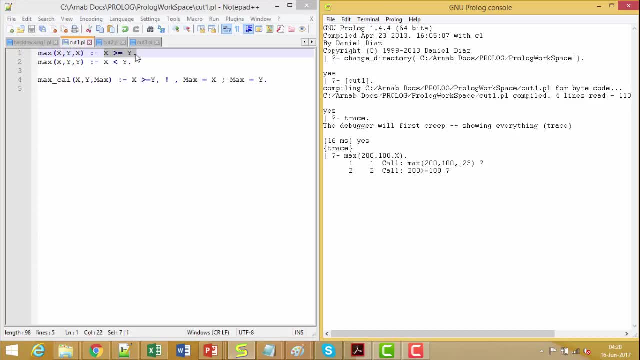 200 is greater than 100, so 200 is greater than equal to 100.. So this condition is true, So it will exit with success, and so this respective variable will be displayed: respective y. the respective x, rather, has been initialized with 200. so in this way you know that. 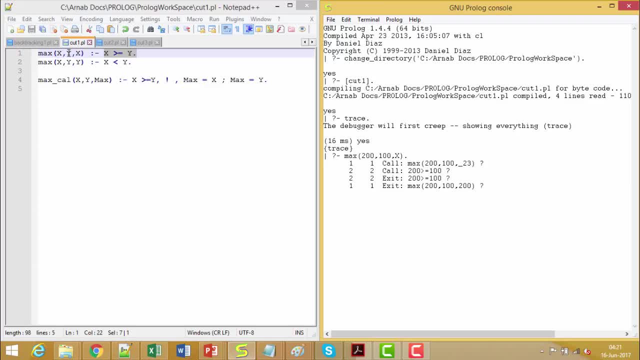 this is my 200, this is my 100 initial initialization, so the last x has got the value 200 accordingly. so here, as we didn't use this cut symbol, so that that's why it is also executing the second clause, which is not at all required. so this is the respective output. so let me put. 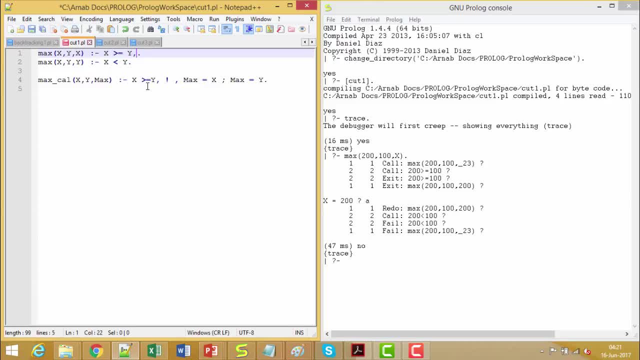 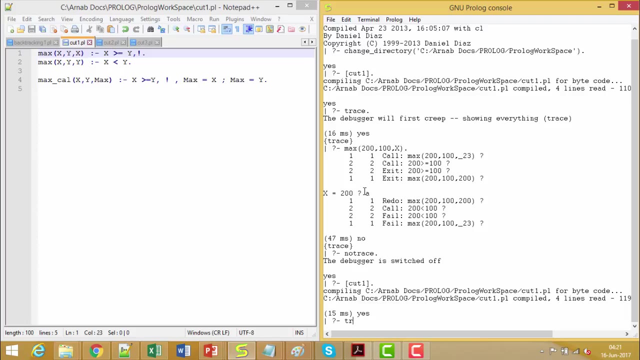 the cut symbol here to show you that how can you get the output faster? so i've saved this one. i'm going for no trace, so i'm just making this cut one on again. i'm making this trace on so so again i'm executing my code. 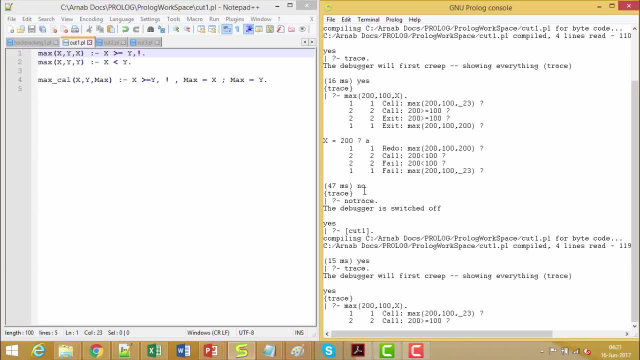 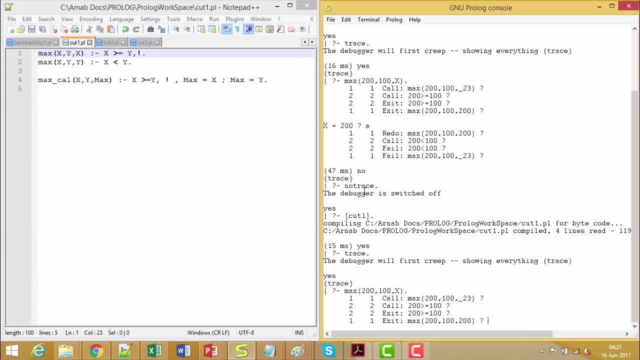 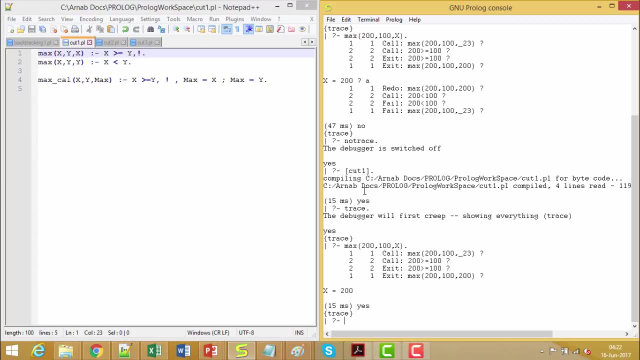 so 200 is greater than equal to 100, it is true. so coming out, exiting with true, so 200 is the maximum. so now you see it is not going for evaluation of the second clause because we have, we are having their cut so when the condition is getting true, so it is coming out, so i'm getting my output faster. 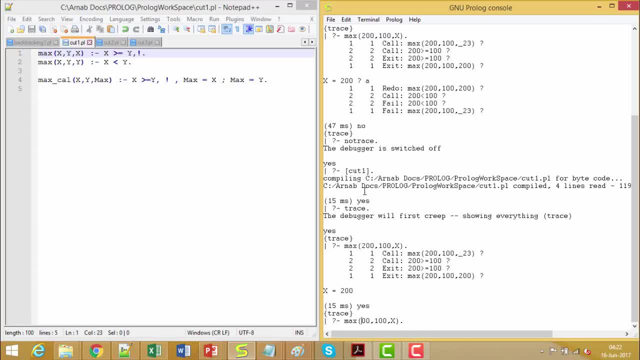 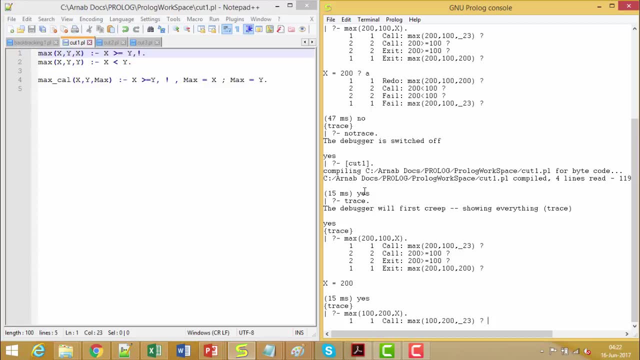 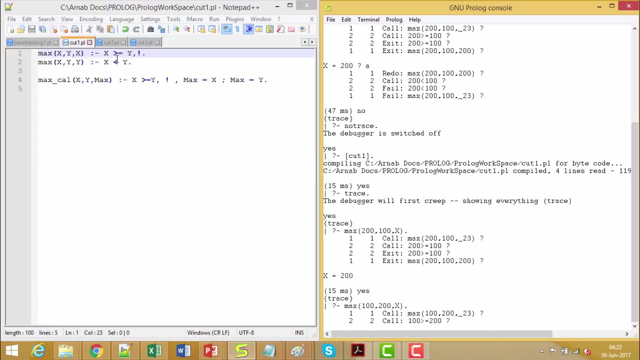 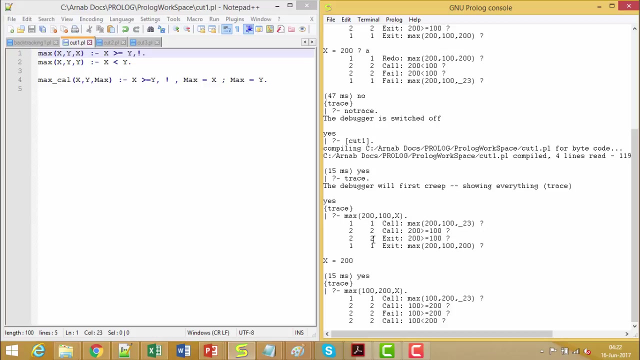 here. so if i make this one as 100 and thiszuf so 100, so the second argument has 200. so 100-200 has been passed as first 2nd arguments. so 100 is greater than equal to 200. so this clause is returning false here. it is fail. so now calling: 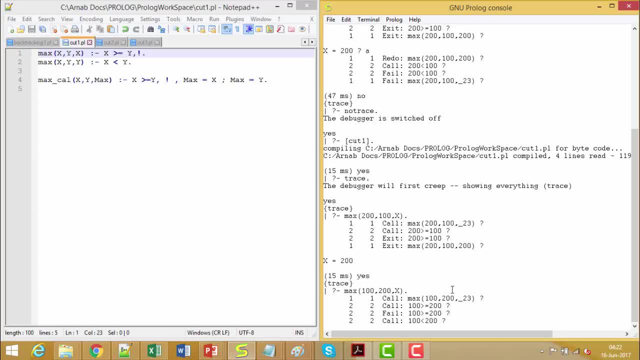 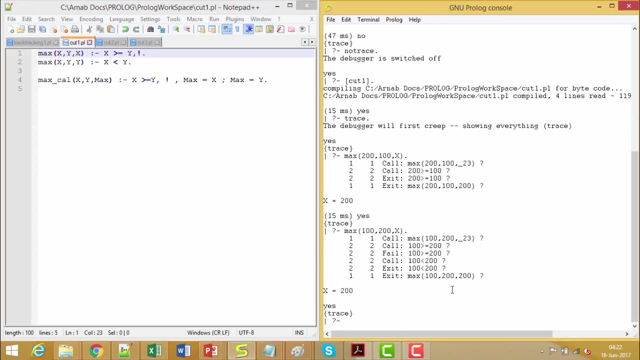 this one, that is, x less than y, is being called, so 100 and 200 are true, so exiting with true. and if complex X less than Y is called, then X less than Y is doing good. oneה and ε is giving us the correct result. so what is happening? you see, we are getting the 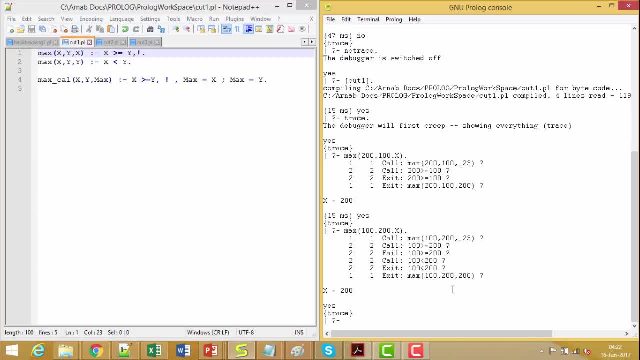 faster result after introduction of the cut symbol. so now let us go for the second predicate. so here we are having this max Cal, so let me execute the same. so I'm going for this with max Cal. so 100 is greater than equal to 200. this 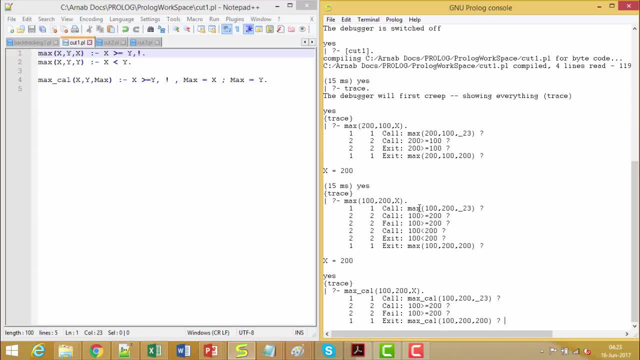 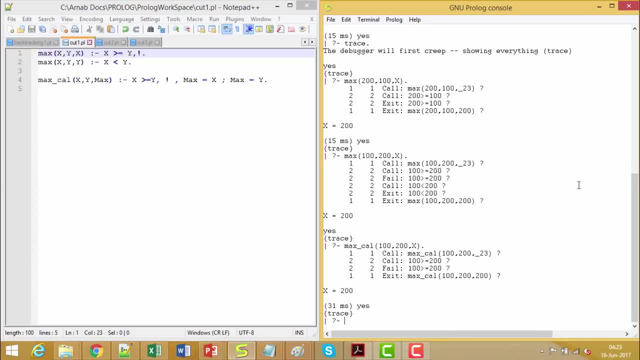 condition is false, so it is fail. so now it is calling this one as 100. 200 is 200, so because here the last, this OR, is getting executed, so that's why we are getting this output. so now let me execute the same, swapping the values of: 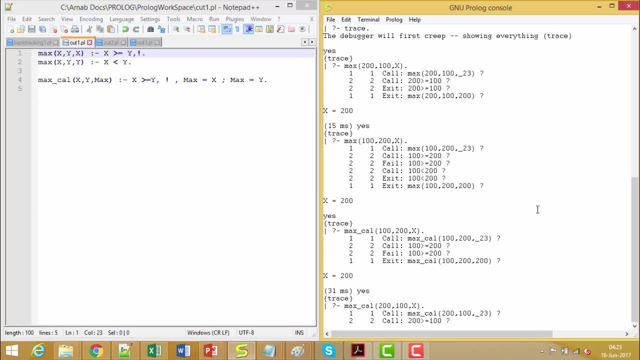 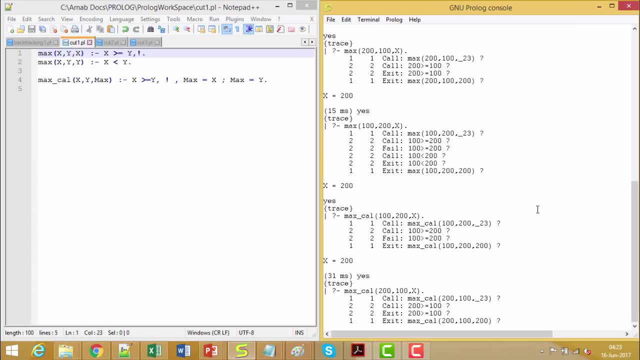 100 and 200. 200 is greater than equal to 100. this condition is true, so it is excellent. so now let us go for the second predicate. so we are having this exiting, so 200 is answer. so this is the use of our cut symbol. thanks for.